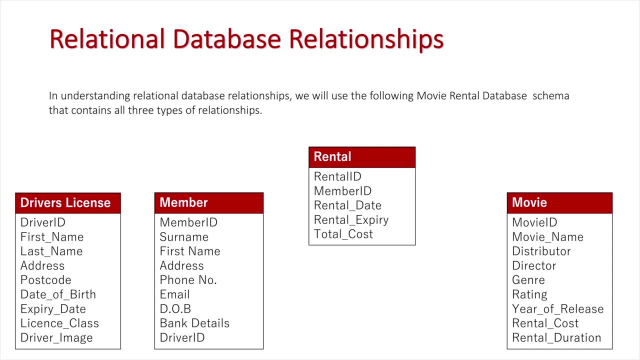 So these are the four entities we're going to be using here to illustrate the three different type relationships of one-to-one, one-to-many and many-to-many. So, firstly, we're going to look at the primary and foreign keys in order to establish our relationships. So the first 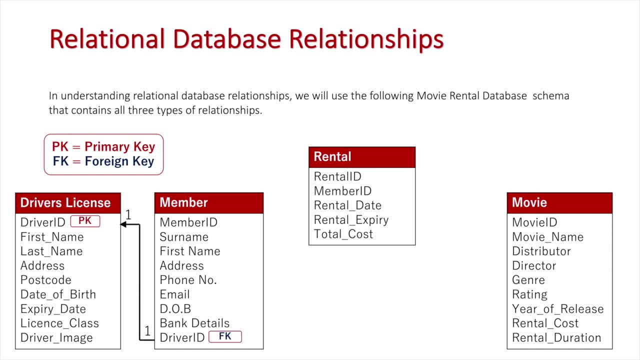 one is a one-to-one relationship between member and driver's licenses. Every member has one driver's license- Okay, that they are going to use to verify themselves, and one driver's license is only going to be used to validate one member- Okay, so it is one-to-one, the records between each other only. 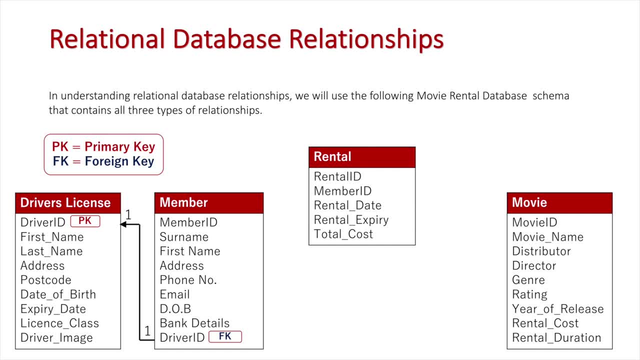 correlate with one another, between those two entities. Next is member and rental, and that is a one member can make many rentals, but every rental only relates to one member. And then, finally, is between movie and rental, and this is a many-to-many relationship. And in order to do that, once again, 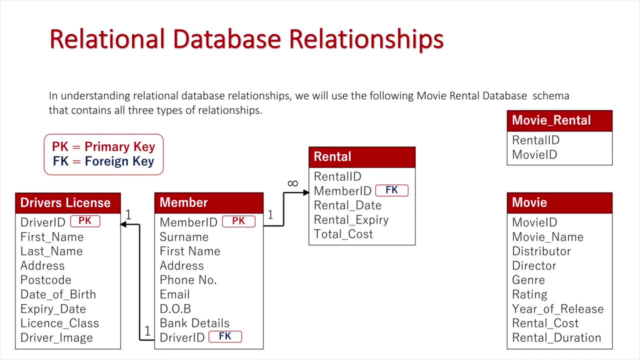 we need a junction, Okay. that junction has two foreign keys within it, Okay, which are both primary keys of each entity involved here. So they are many-to-many relationship, as one movie can refer to multiple rentals and every rental can refer to multiple movies. in order to establish that, 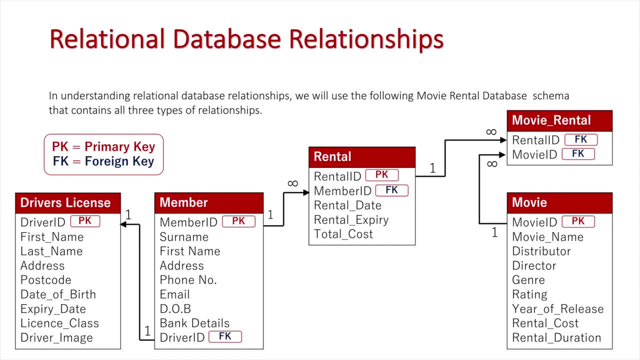 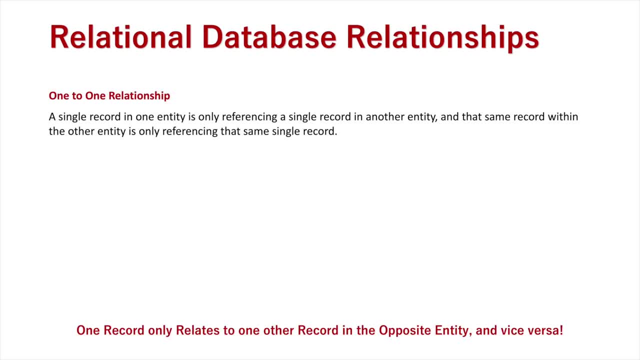 relationship. So we've said the relationships, we've shown them in a schematic design, but let's have a look at what those relationships actually look like when we're referring to records, because these are all based on records referring to each other. So firstly is the one-to-one relationship. 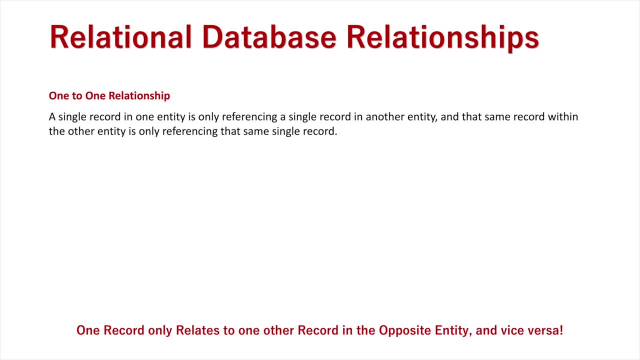 where a single record in one entity is only referencing a single record in another entity and that same record obviously is only referencing it in return. So let's look at members and drivers licenses. So between member and driver's license: okay, member ID 2 is only referencing driver ID 2.. 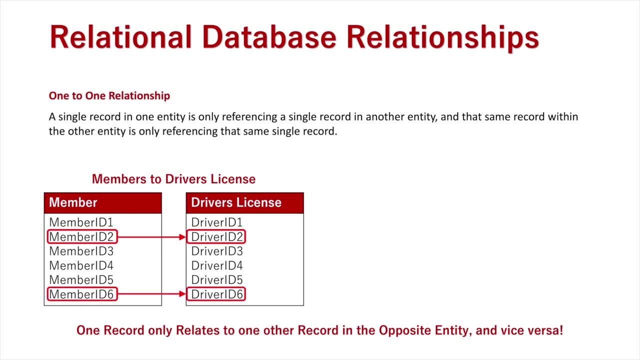 And member ID 6 is only referencing driver ID 6.. Okay, it only references one record in the opposing entity, On the flip side of that of driver's licenses to members. it's exactly the same, Okay. driver's ID 2 is only doing member ID 2.. Driver ID 6 is ending member ID 2.. So it's exactly the. 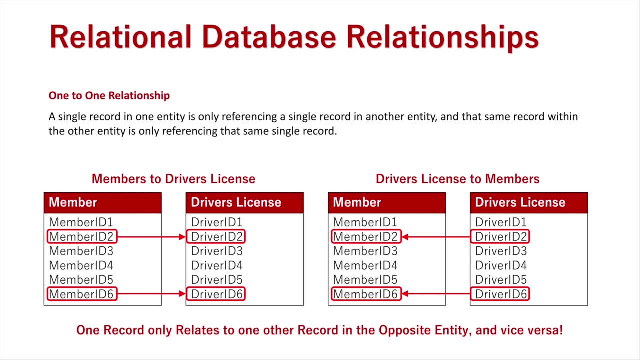 same, going both ways. One record one only references one in the other. Okay, exactly the same way it is. It is a simple relationship. Okay, one record only referencing one other record. Next is the one-to-many relationship or the many-to-one relationship. Okay, where a single. 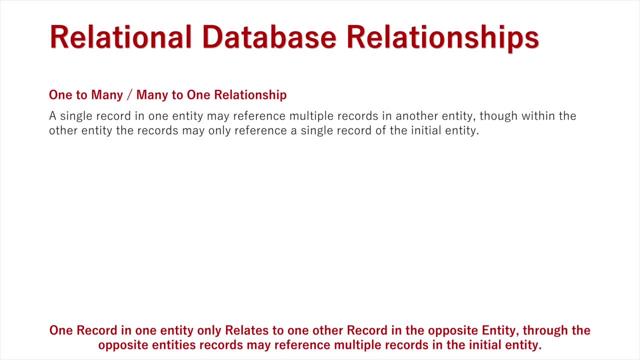 record in one entity may reference multiple records in another entity, though within the other entity the records may only reference a single record in the initial entity. So, as we've already stated, member-to-rentals okay is a one-to-many relationship, Okay, so one member. 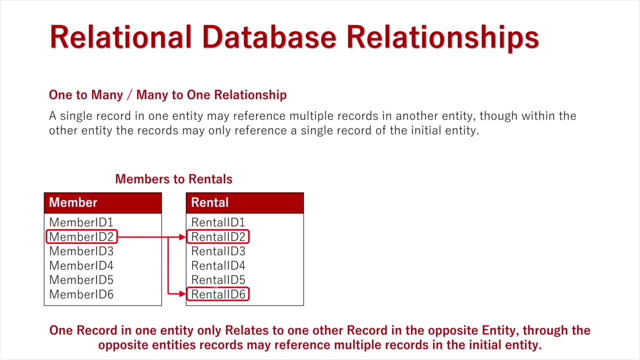 okay, member ID 2 might make multiple rentals. So rental ID 2 and rental ID 6 might both refer to member ID 2.. Okay, one person has made two separate rentals. Okay, another example is a member ID 3.. They might have done the rental ID 3 and rental ID 4 and rental ID 5.. Okay, so those three records. 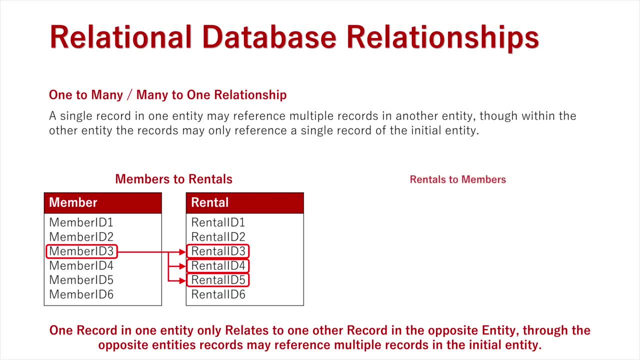 refer to that one specific member, Okay. but on the flip side of that, when going rentals back to members, Okay, we know that rental ID 2 only refers to member ID 2. It doesn't refer to any other member because only one rental can be made by one member. 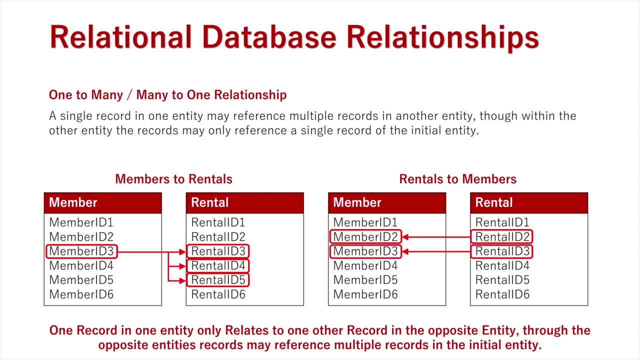 It's the same with rental ID 2. It only references member ID 2.. Okay, so that justification. so it can only reference one record in that entity, but the member entity can reference multiple records in the rental entity. Okay, so that's what we've got to understand with a one-to-many relationship. 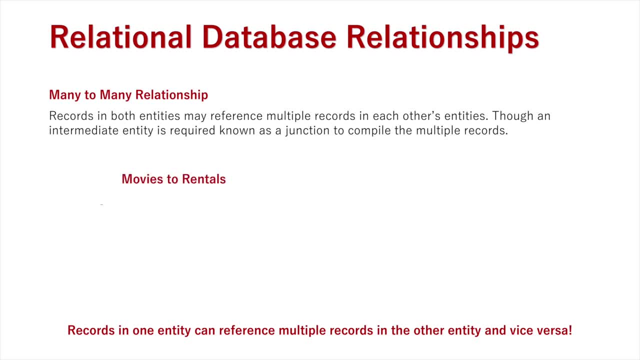 Finally, we have the many-to-many relationship and, as we've already said, movies to rentals was our many-to-many relationship. So movie ID 2 might be used in rental ID 2 and rental ID 6. Okay, and movie ID 3 may be used in rental ID 3 and rental ID 4 and rental ID 5. Okay, so it is going from. 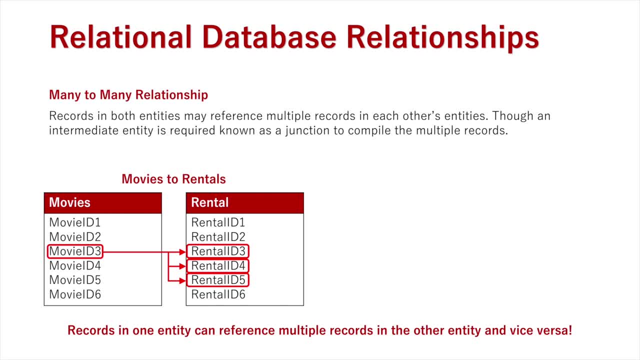 the movies to the rentals, one-to-many, but we've said it's exactly the same on the flip side. Okay, in rental IDs, the movie, and this is why we had to have the junction. So going back the exact opposite way: rental ID 2.. Okay, it might have involved movie ID 2 and movie ID 3. Both those. 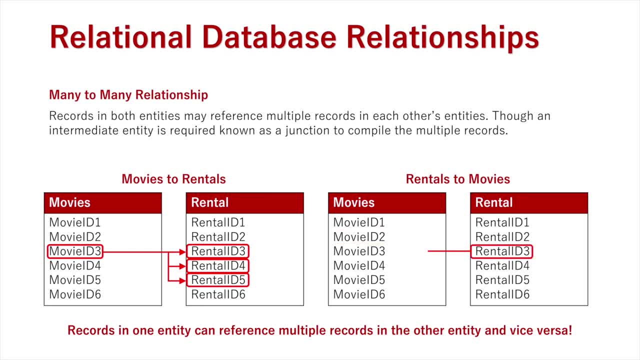 movies were rented during that rental, and rental ID 3 could reference movie ID 2 and movie ID 5.. And movie ID 3 as well goes exactly the same, but also movie ID 4 and movie ID 5.. Okay, so both entities can reference multiple records in the other entity, thus establishing their many-to-many.